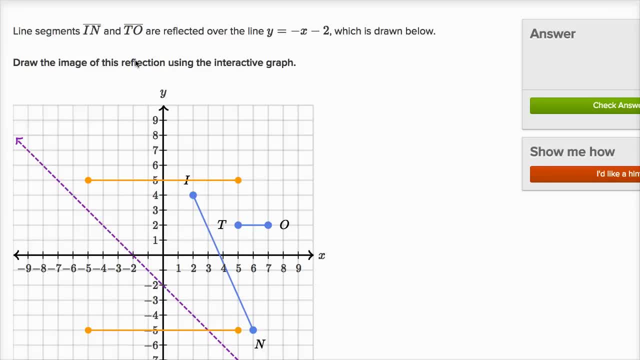 Line segments IN- this is segment IN over here, and TO- this is TO here- are reflected over the line. Y is equal to negative X minus two. So this is the line that they're reflected about, this dashed purple line, and it is indeed 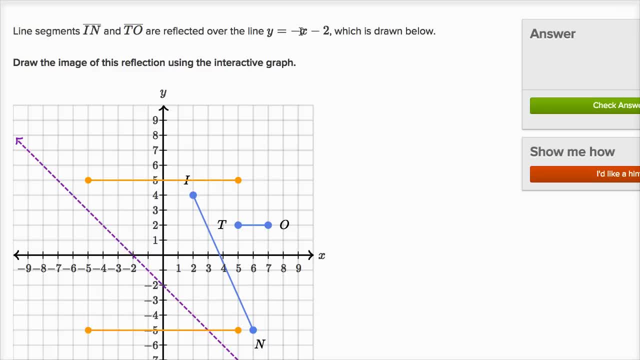 Y equals negative X minus two. This right over here is in slope-intercept form. The slope should be negative one, and we see that the slope of this purple line is indeed negative one. If X changes by a certain amount, Y changes by the negative of that. 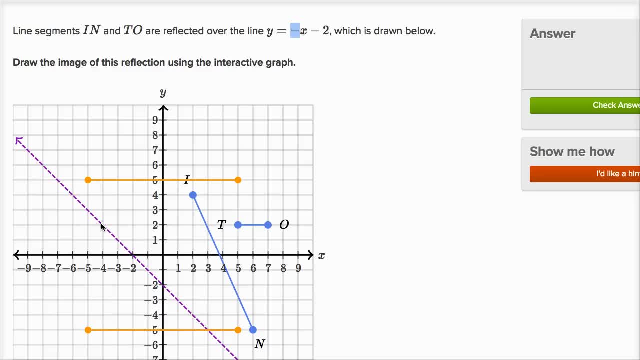 If X changes by one, Y changes by negative one. to get back to that line. If X changes by positive two, Y changes by negative two. to get back to another point on that line And the Y-intercept we see when X is equal to zero. 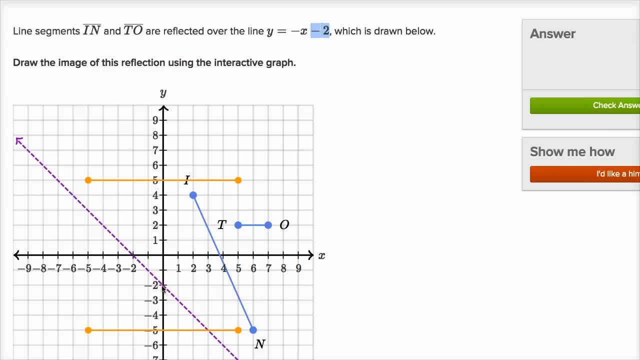 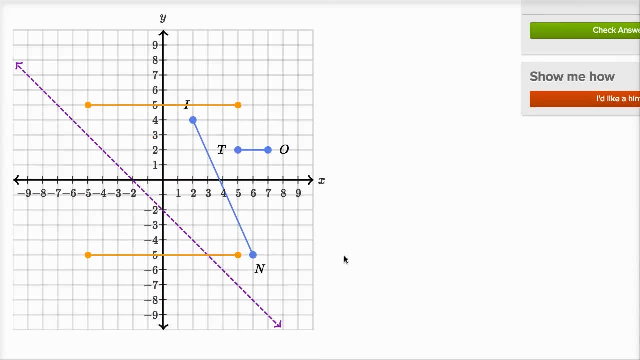 Y should be negative two. When X is equal to zero, Y is indeed negative two. So we validated that. Now they say: draw the image of this reflection using the interactive graph. All right, so we can move these lines around and we want to reflect these. 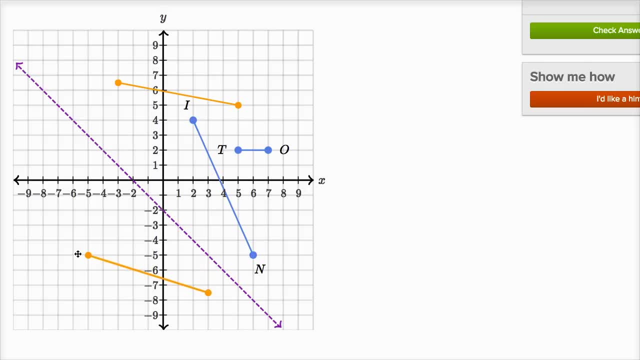 And I could try to eyeball it. you know, maybe it's something like this. I don't know. this doesn't seem exactly right. That looks close to the reflection of I-N And for T-O. I'd want to move this down here. 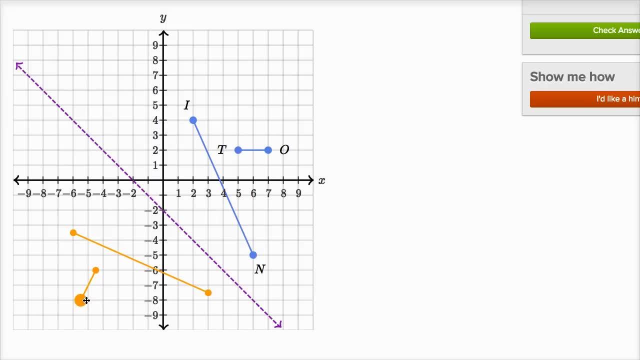 T-O. looks like it would be. I don't know I'm eyeballing it. This is close, but I can't be close. I want to get exact. So let's. I've copied and pasted the original problem on my scratch pad so we can find the exact points. 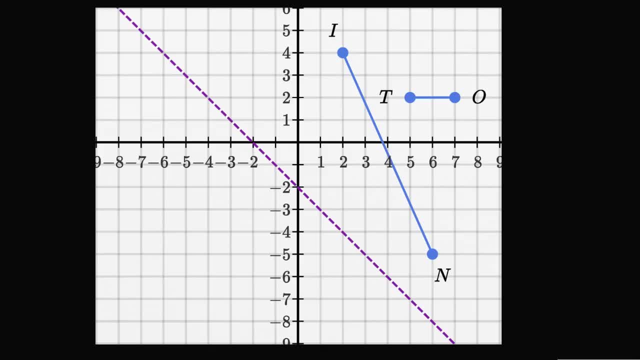 and so I don't just have to estimate this. So let's go to the scratch pad. So exactly what we just saw, And the main realization is is, if we want to reflect a given point, if we want to reflect a given point, 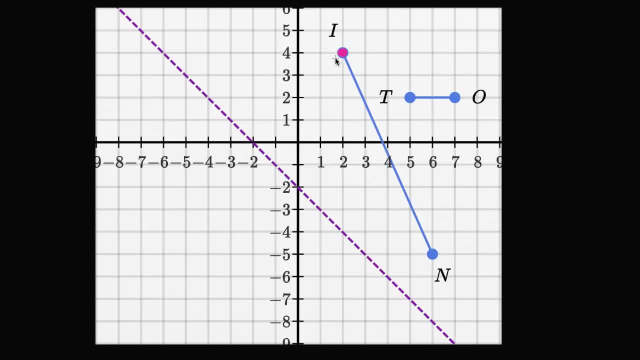 say point I right over here. what we want to do is we want to drop a perpendicular. We want to find a line that's perpendicular, a line that has the point I on it and it's perpendicular to this line right over here. 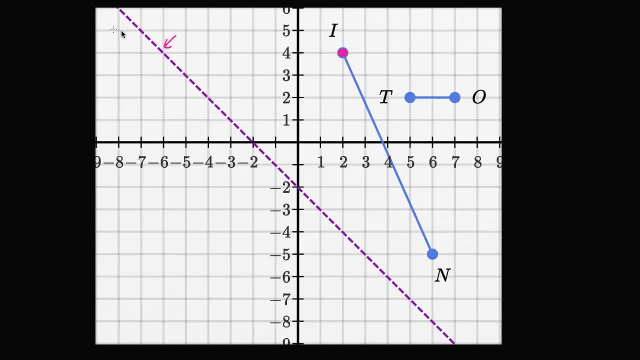 Remember, this is the line. let me do this in that purple color. This is the line: y is equal to negative x minus two. It's slope, it's slope is equal to negative one. So I want a line that goes through. I point. I. 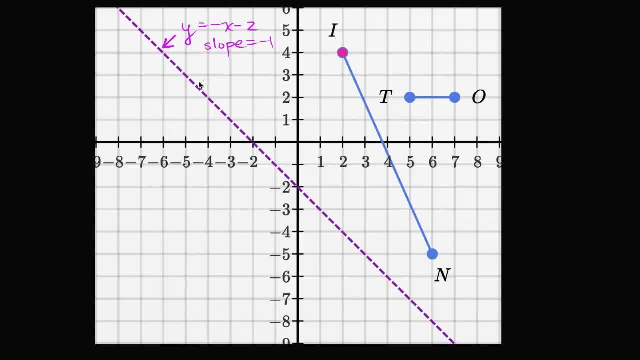 that has a that is perpendicular- perpendicular to this line- and I want to drop it. I want to drop it to. I want to drop it to the line that I'm going to reflect on, and then I want to go the same distance. 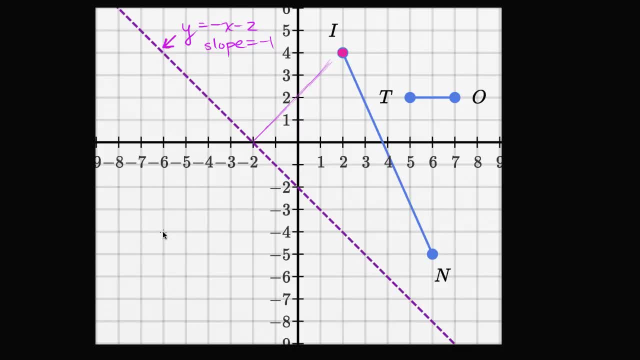 onto the other side to find, to find the corresponding point in the image. So how do I do that? Well, if this line, if this purple line, has a slope of negative one, a line that is a line that is perpendicular to it, 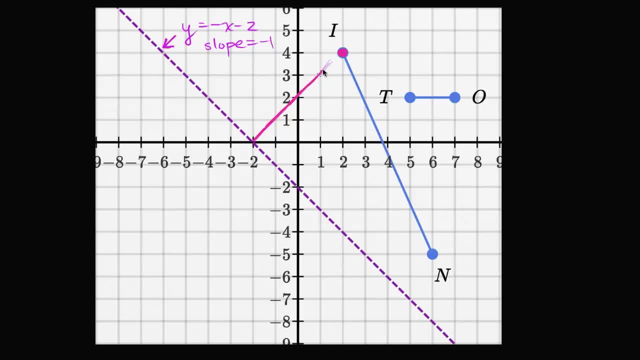 so this thing that I'm drawing in purple right over here, its slope, is going to be the negative reciprocal of this. So the reciprocal of negative one is still just negative one. One over negative one is still negative one, but we want the negative of that. 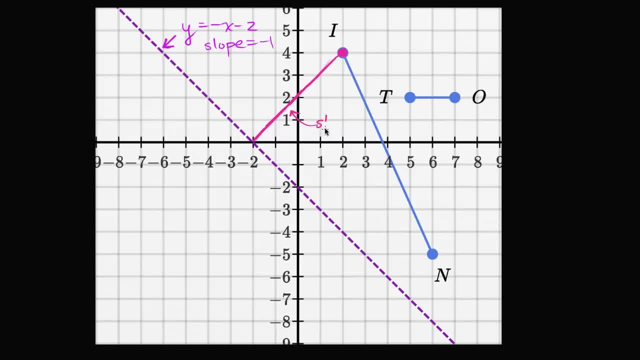 So the slope here needs to be one, and luckily that's how I drew it. The slope here needs to be equal to one, which is: however much I change in the x direction, I change in the y direction. We see that To go from this point to this point right over here, 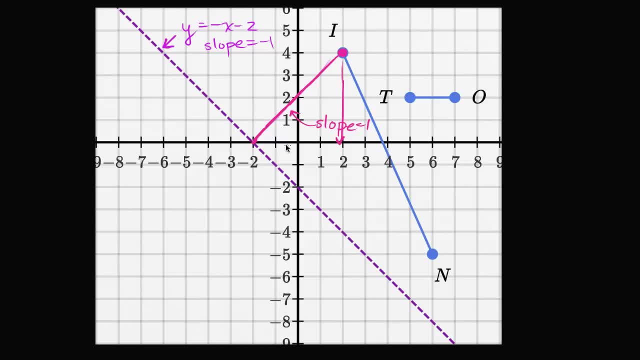 we decrease y by four and we decrease x by four. Now, if we want to stay on this line to find the reflection, we just do the same thing. We could decrease x by four, so we'll go from negative two to negative six. 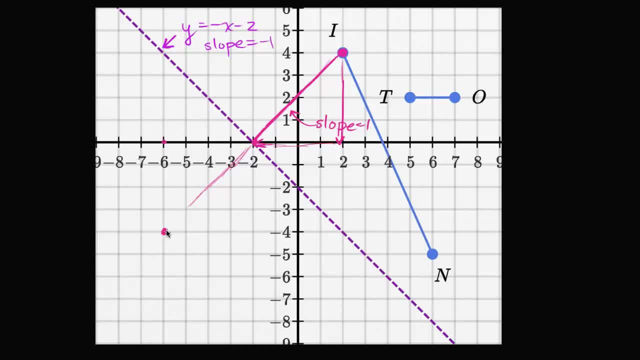 and decrease y by four, and we end up at this point right over here. So we end up at the point this is: x equals negative six, y is equal to negative four. So this is this point corresponds to this point right over there. 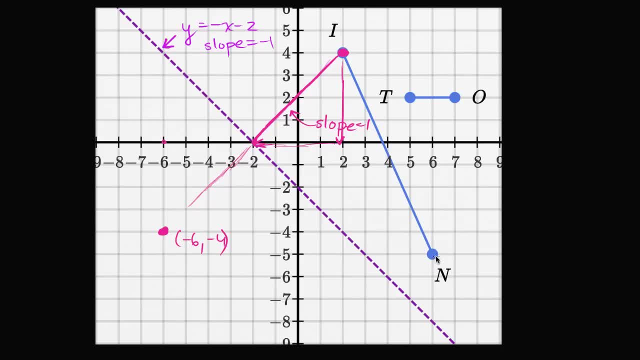 Now let's do the same thing for point n. For point n, we already know: if we drop a perpendicular, if this is perpendicular, it's going to have a slope of one, because this purple line has a slope of negative one. The negative reciprocal of negative one is positive one. 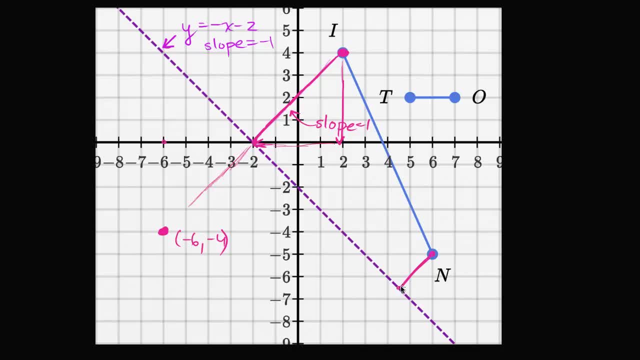 And let's see, to go from this point to this point of intersection, we have to go down one and a half, we're going down one and a half and we're going to the left one and a half, So we want to do that on the other side. 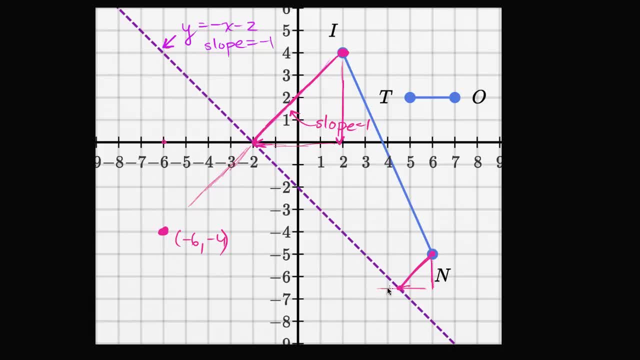 We want to stay on this perpendicular line, so we want to go left one and a half and down one and a half And we get to this point right over here, which is the point x equals three, y is equal to negative eight. 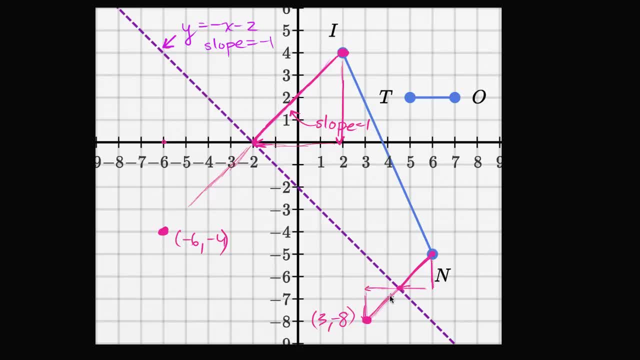 And so we are now equidistant. we're on this perpendicular line still, but we're equidistant on the other side. So the image of i? n is going to go through negative six comma negative four and three comma negative eight. 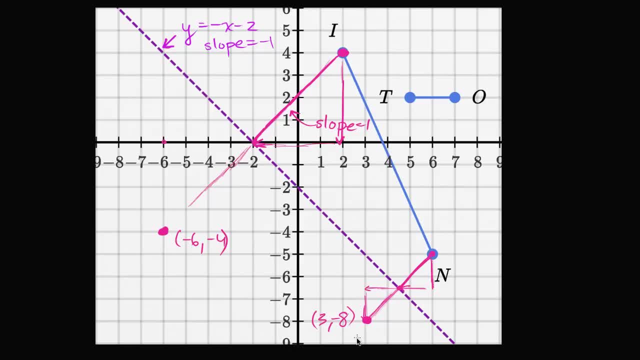 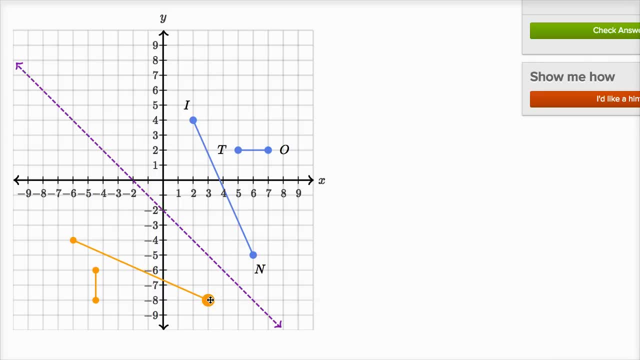 So let me draw that And remember: negative six: negative four, three comma negative eight. So I have a bad memory. So negative six, negative four and three comma negative eight. And I was close when I estimated but I wasn't exactly right. 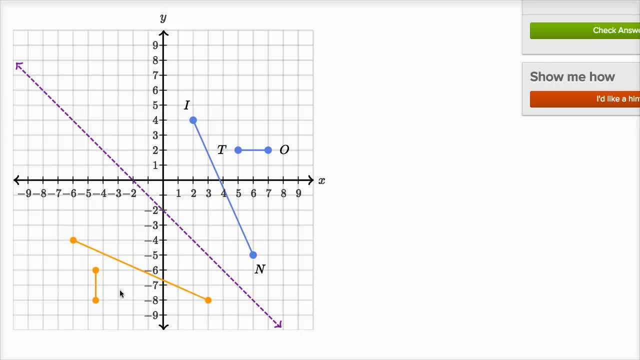 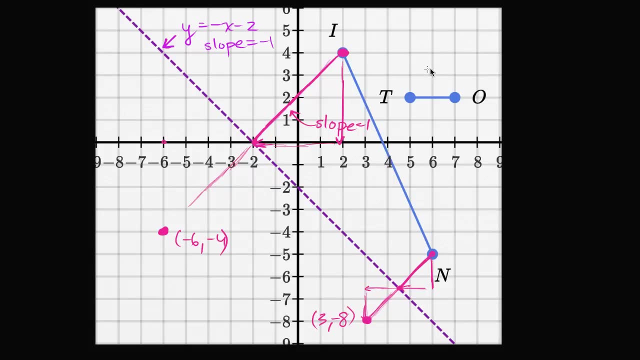 So that's looking pretty good. And then actually we can do the exact same thing with points t and point o, And let me do that. So point t: to get from point t to the line in the shortest distance. once again we drop a perpendicular. 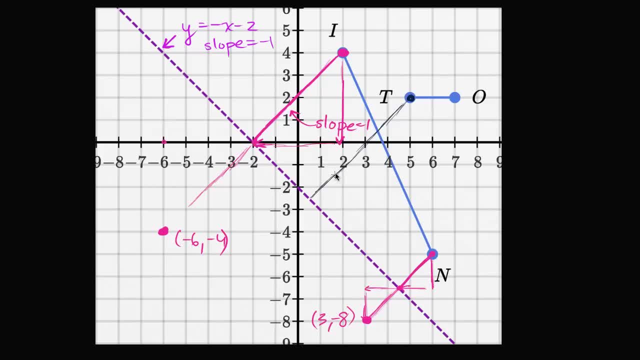 So the line is going to have a slope of one, because it's perpendicular to the line that has a slope of negative one. And so, to get there, we have to decrease our x by we have to decrease our x. we're going from x equals five. 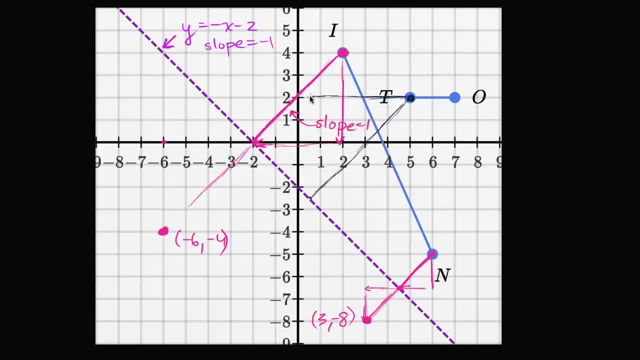 to x equals looks like half. So x went down by four and a half in the x direction and y also needs to go down by four and a half. So if we want to stay on that line, let's decrease our x by four and a half. 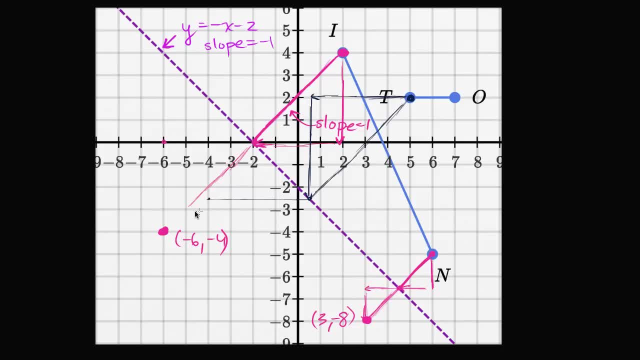 so that's half one, two, three, four. and y needs to go down by four and a half. So that's half one, two, three, four. and we get to this point right over here, which is the point x equals negative four. 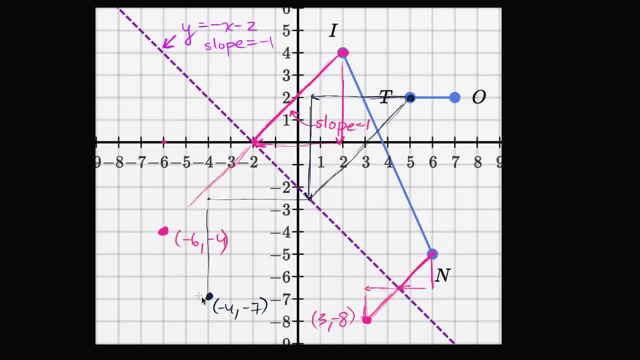 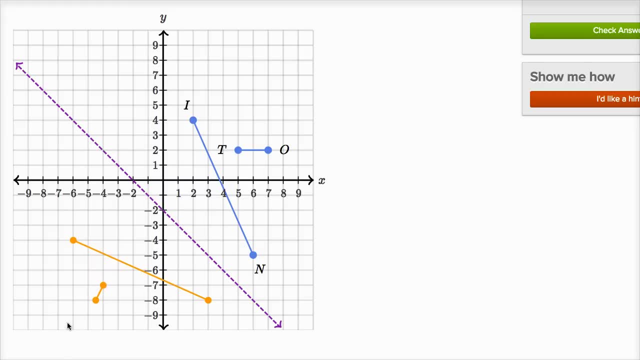 y is equal to negative seven. Negative four. comma: negative seven. let me so this should be at: x equals negative four, y equals negative seven, And there's a couple of things you could do here. You could just say this is too long. 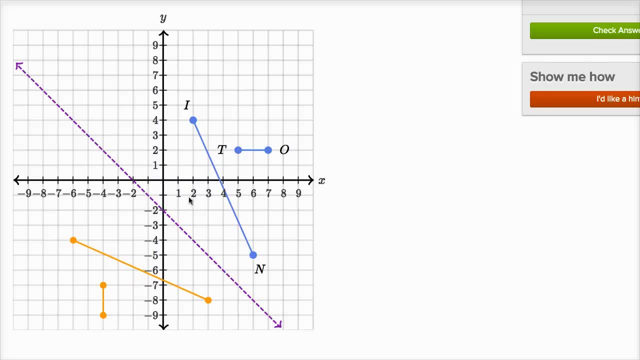 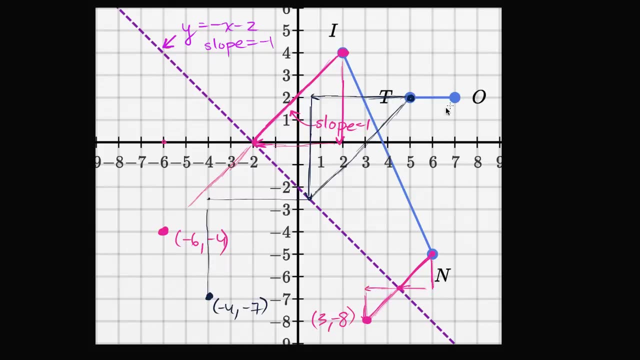 or two units long, not like too long in length somehow. This is two units long, so maybe this is two units long. So this is feeling good, Pretty good. But let's just go through the exercise for point O as well. So point O. 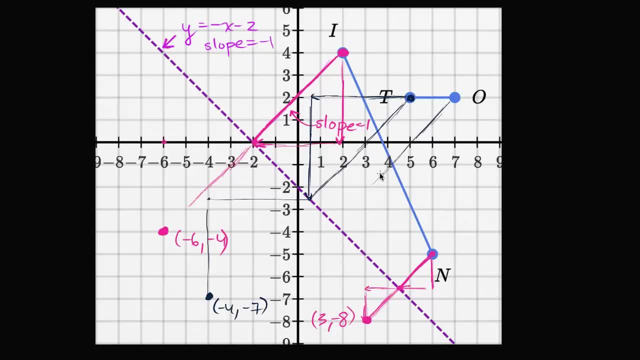 once again this is going to have: if we drop a perpendicular, it's going to have a slope of one. So, whatever our change in x, between this point and this point, we're going to have the same change in y And our change in x to go from seven to. 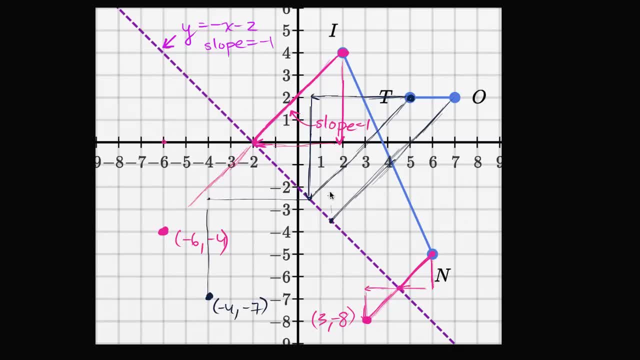 seven to one and a half. our change in x is five and a half, So maybe let me do it this way. So the change in x here the change in x is equal to negative five and a half, 5.5..